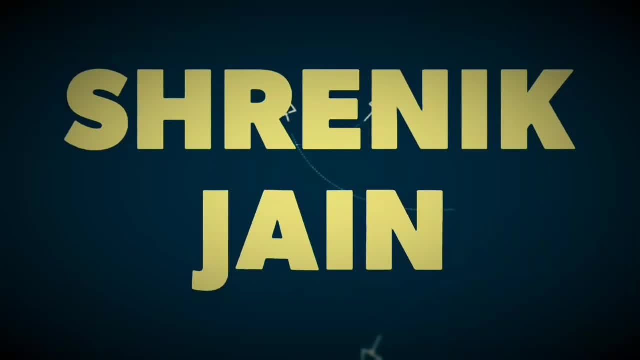 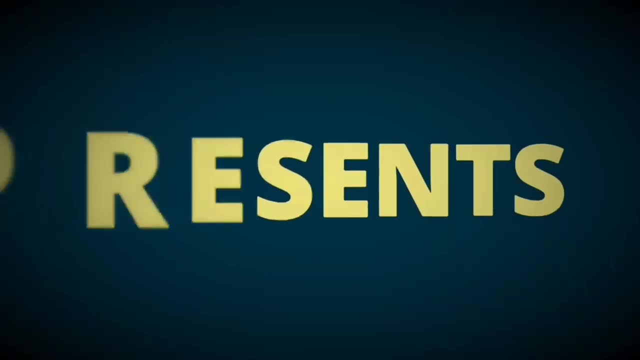 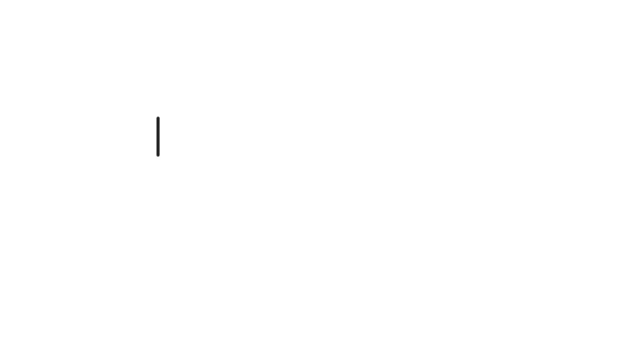 Hello friends, today our topic is Binomial Distribution. So first we will see the formula. So p of x equal to small x, that is, ncx. p raise to x, q raise to n minus x. Now let's understand the terms of the formula. So our first term: 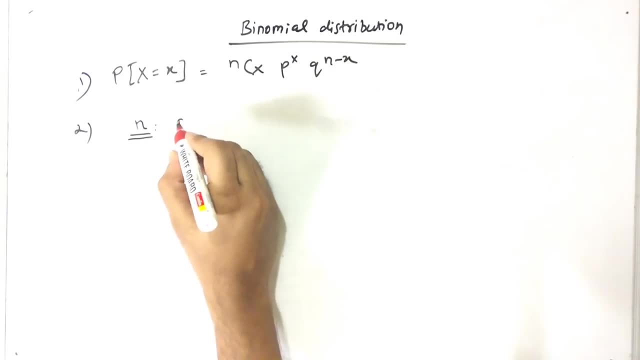 is n. Now, n means it's a finite value and it is always the total. Example: we can have 1000 books, So our n is 1000.. Similarly, there can be 10 pens or 15 bulbs, So these are nothing but n. Our second term is p and third term is q. 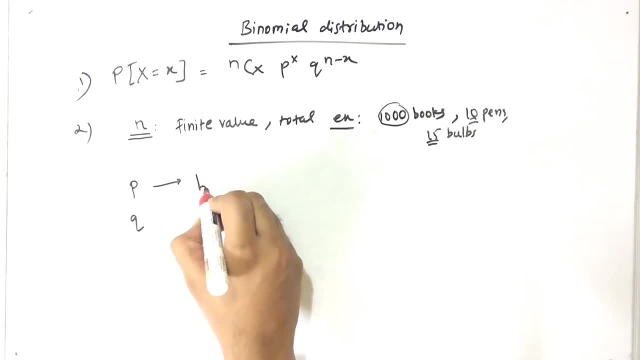 So p always meant success, whereas q means failure, And the relation between these two is p plus q equal 1. Now x. x means this term. we have to find it from quotient and it is present in last line of the quotient, So let's understand. 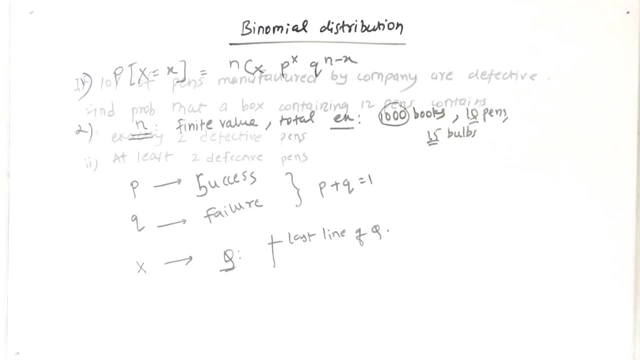 this by an example. So the question is: if 10% of pens manufactured by any company are defective, then find the probability that a box containing 12 pens contains exactly 2 defective pens. Second question is: at least 2 defective pens Exactly? 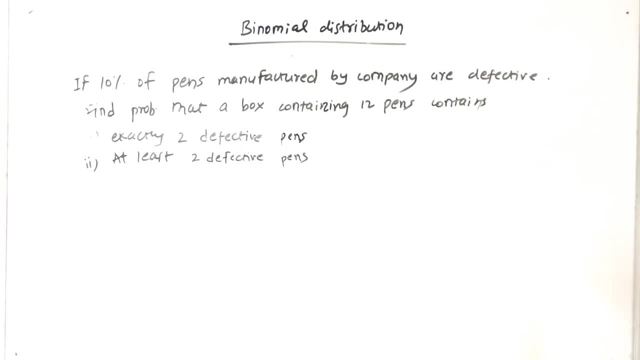 means equal to 2.. At least means 2 and more. So let's see how to solve this. First we have to find the parameters. So the first parameter was n, and n means the total number. you can see: total is 12 pens, so n is equal to 12. second was to find p. now here, p means 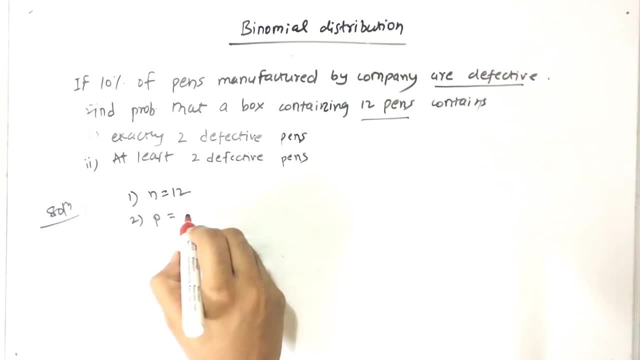 the pens are defective, so p means defective and the probability is 10 percent, so 10 by 100, that is 1 by 10. then what is q? q is 1 minus p, that is 9 by 10. now we have our basics, like NPQ, we have 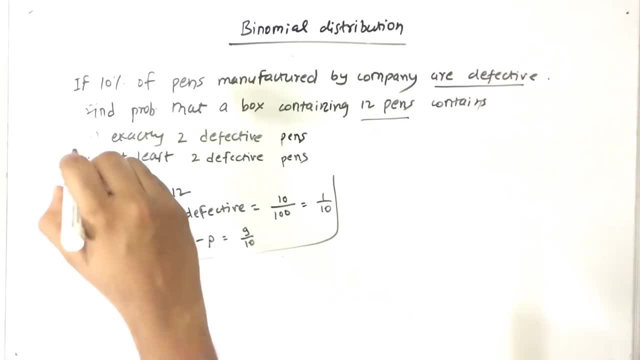 now we need X. now X was from the question, so we have two, question one and two. so first question: we have to see p of X equal. now here exactly two pens are defective, so X value equals 2. now substitute in the formula. the formula was NCX, p raised to X, q raised to. 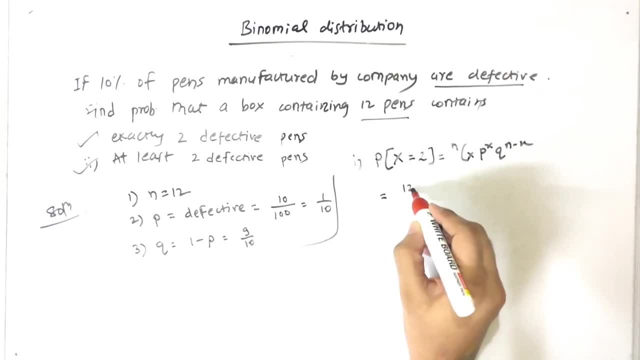 NCX, p raised to X, q raised to NcX, ncX, p raised to x, q raised to NcX minus X. so n is 12, see X is 2, P is 1 by 10, again X is 2, Q is 9 by 10 and n minus. 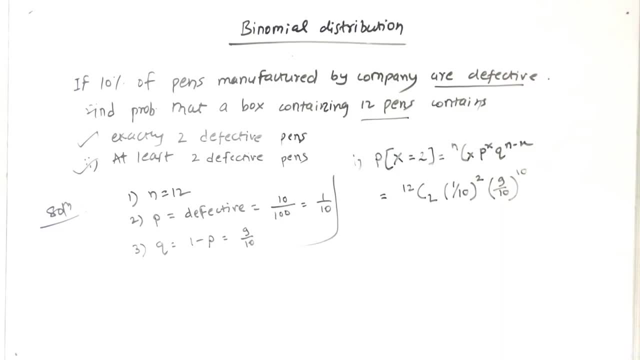 X is 2 or minus 2, that is, 10. after solving this you will get the answer. now talking about the second condition. the second condition is: at least two defective pens. now at least means P of X. first. it should be equal and greater, so greater than equal to 2, which is nothing but 1 minus P of X, less than 2. 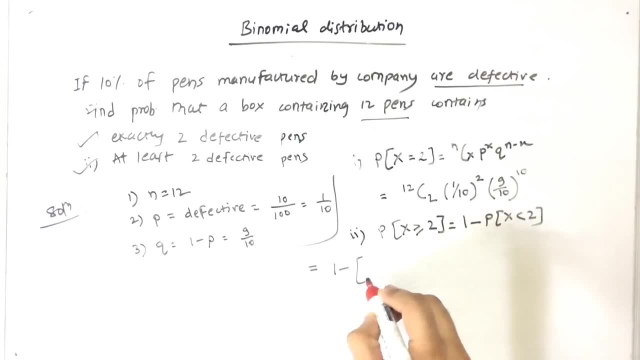 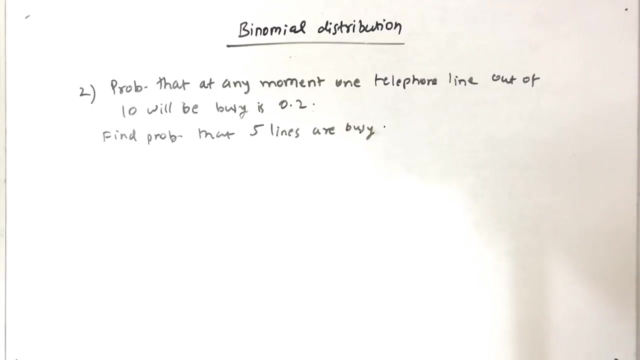 now it can be written as: 1 minus P of X, equal 0. plus P of X, equal 1. let's take another example. so the example 2 is: probability that at any moment one telephone line out of 10 will be busy is 0.2. find probability that five. 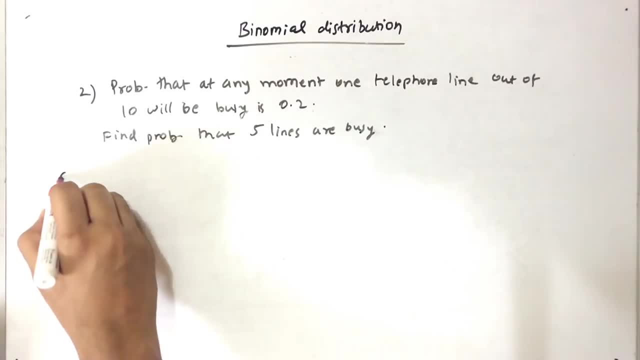 lines are busy. now first we have to find the parameters n, P and Q. and means the total. so there are total ten telephone lines. P means the probability. now here we consider P as the busy, so the probability of line being busy is 0.2. so what will be Q? Q is 1 minus P, that is 0.8. so we are done. 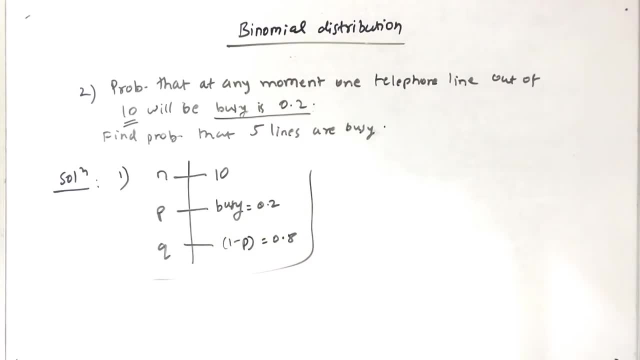 with step 1, that is, finding the terms for the formula. second is, what is the condition that is finding X? now the question is this: find probability that five lines are busy, so P of X equals 5, and now, using the formula that is, n, C, X. 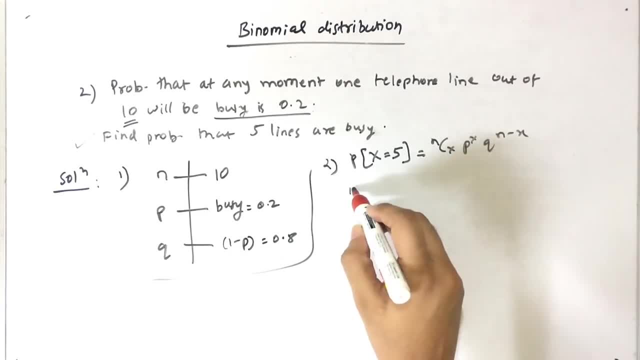 P raised to X, Q raised to n minus X, n is 10 C, X is our 5, probability is 0.2. again, X is 5, Q is 0.8 and n minus X is 10 minus 5. after solving this, we get the answer. 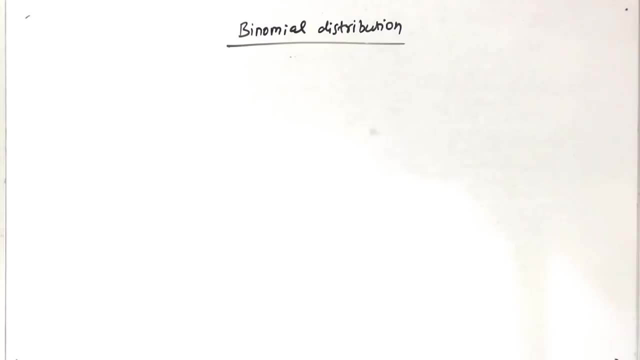 now let's see the properties of binomial distribution. so the first is expected value, or it is also called as mean. that is nothing but n into P. now second, second day, variance. we get this represented as sigma square, that is NP, Q. so standard deviation is routine. so the difference between Bernoulli and binomial. 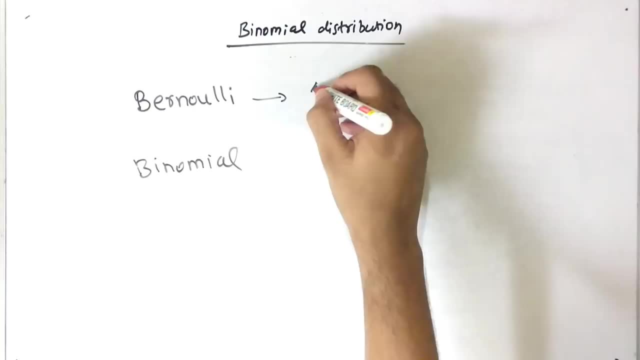 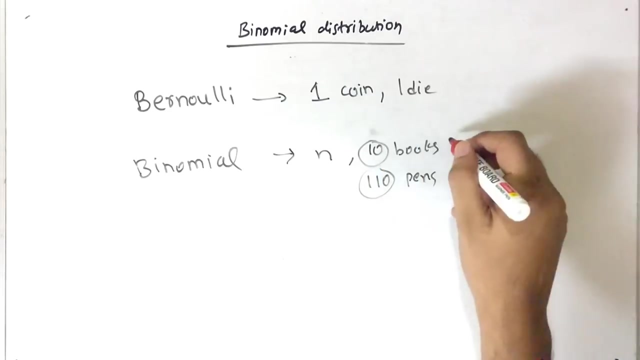 distribution is simple. that Bernoulli was for one, like one going one dye to for a coin or for a dieatz flight. it was very simple, like it, for it was for one. but binomial is for n, like 10 books or let's say 110 pence. that's why the term n in binomial is very important. 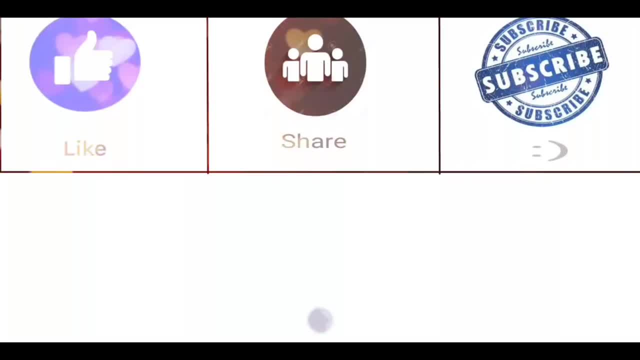 so, friends, if you like my video, then do like this video, share with your friends and subscribe to my youtube channel so meet you in next video. till then, take care, this is shrenik jain. peace out.